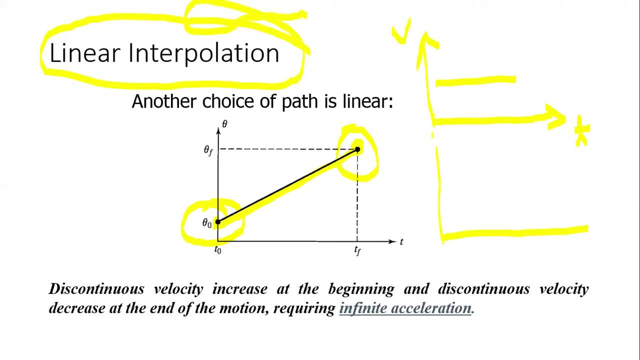 type of velocity and the acceleration will be like this: an infinite acceleration, then suddenly zero and negative, infinite deceleration. this, this much acceleration, is not possible for any kind of actuator. so this limitation makes this approach very difficult, if we don't add something at the beginning and at the end. so to tackle this problem, what we do, we add a. 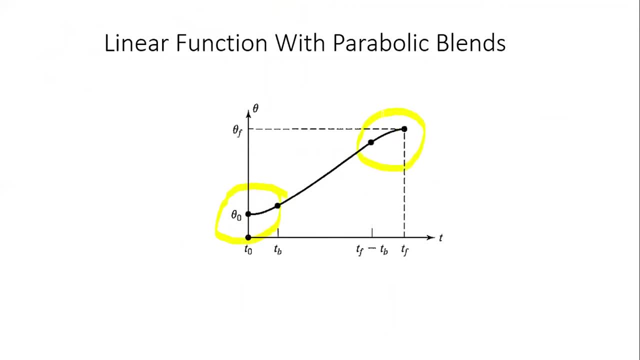 parabolic blender at the beginning and at the end. so with the addition of these parabolic blends we make the acceleration at the beginning and deceleration at the end to a limited or to a defined value. so for these two segments we get constant acceleration if we use parabolic. 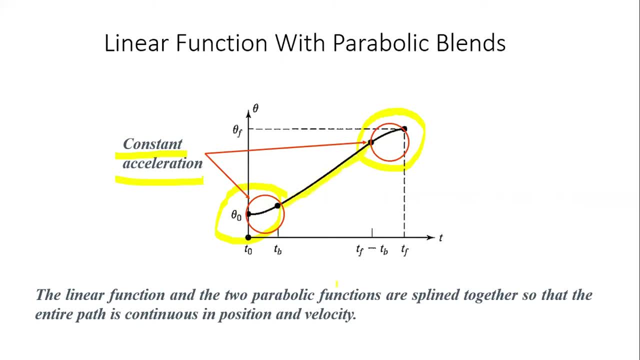 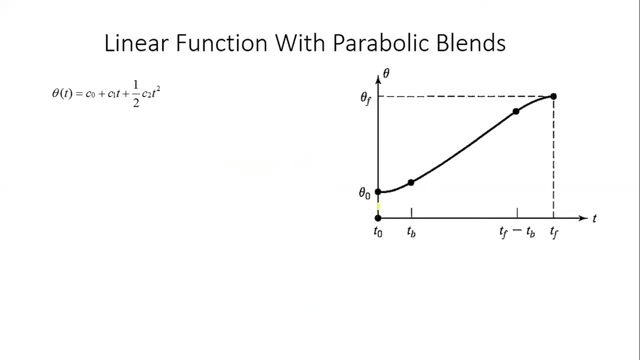 the linear function from this point to this point, and two parabolic function, one and one here are splined together so that the entire path is continuous in position and velocity. okay, so this linear function with parabolic blend can be described by this equation. so if you take the first order, derivative of this equation, you 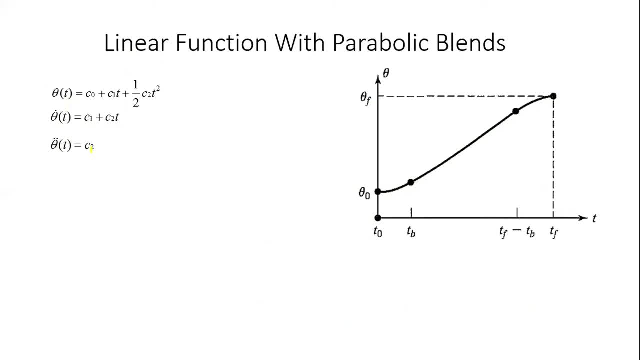 will get t dot. t is equal to c1 plus equal to t and theta double dot is equal to c. so initially at t is equal to 0, the velocity is 3 and at t is equal to 0. so at another point we see that it is. 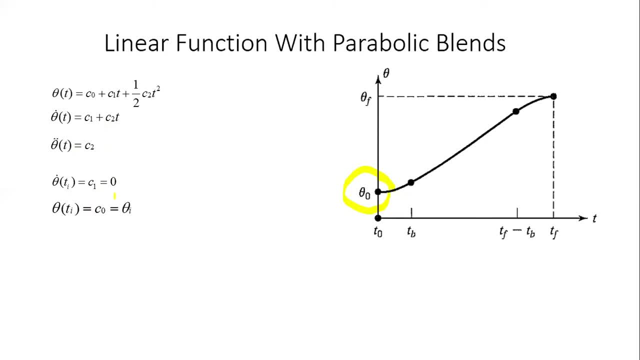 going to be a constant acceleration. so i will explain that with this, how we will know what the equation is for a simple exercise, and then i will explain this in detail so you can understand. the t is zero, so c1 will be equal to t. at t is equal to zero, the position is theta zero or theta initial. 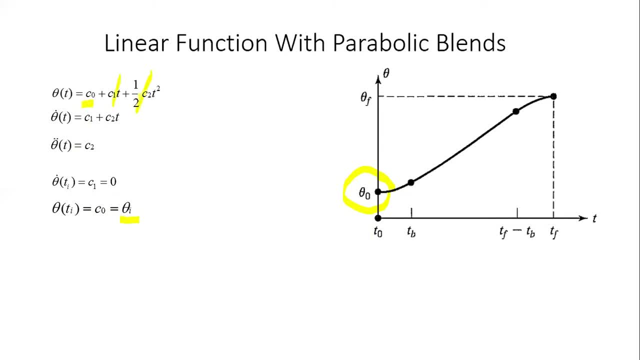 theta i. so c naught. by putting t is equal to zero, we will get theta i is equal to c naught. so after substituting all these constraints in this expression, we get: theta t is equal to theta i plus half c2 t. c2 t squared it gives theta dot c is equal to c2 t and theta double dot t is equal. 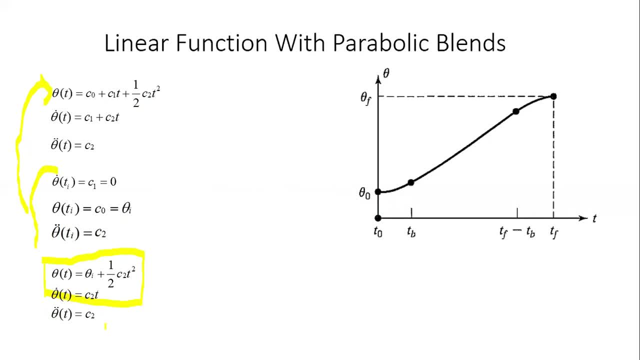 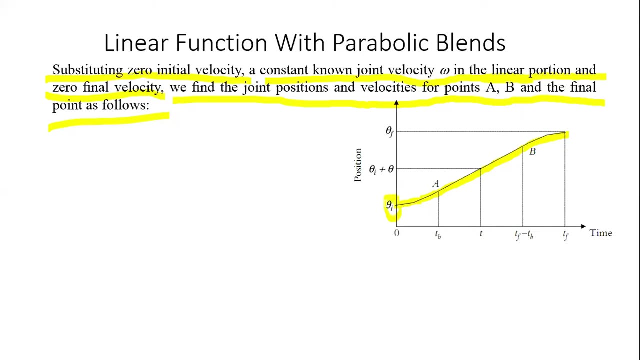 to c. then the question arises that how to? how to find this time tb and the corresponding position of the profile? so for that we follow this procedure. we have divided the trajectory into several segments, so at this point the velocity is assumed to zero and the velocity in linear 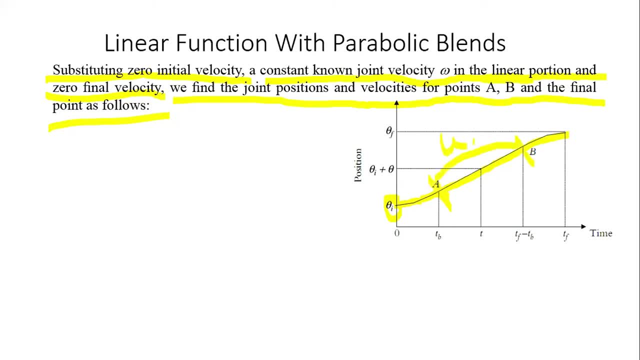 segment from here to here is assumed omega and the velocity at the final position is assumed zero. so with these boundary conditions, we can find out the joint positions at point a and point b and also the velocity at point a and point b. okay, so using the previously derived expression, 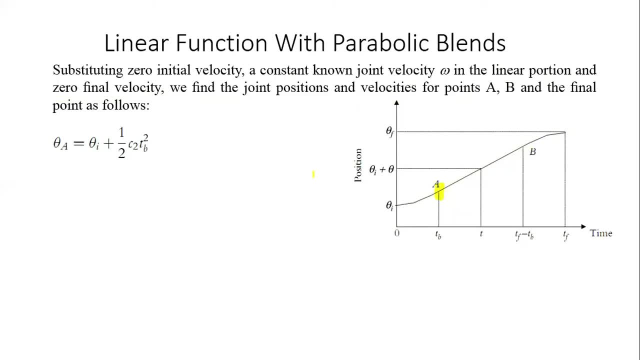 we can find out the expression of position at point a and it will be: theta a is equal to theta i plus half c2 tb squared, a derivative, and we will get theta i. dot is equal to c2 tb is equal to omega, because omega is constant. 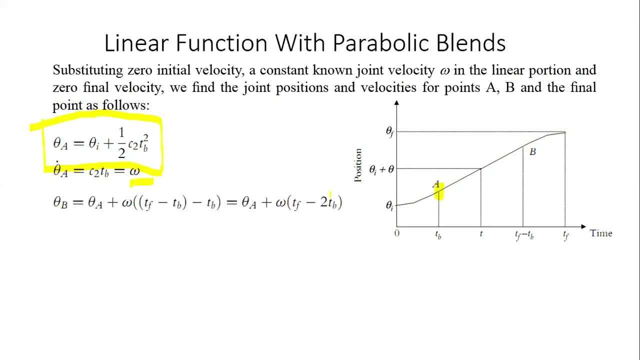 from the point a to point b. at point b the position can be represented by theta b minus theta a by the time difference from here to here. so if we divide this theta b minus theta a by this time difference, then this will give us the angular velocity. for me, this equation has been 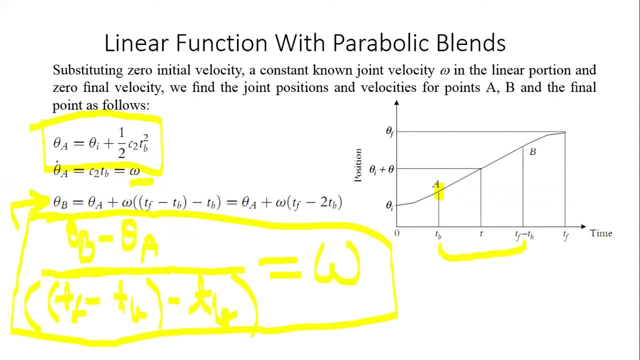 written like this: theta b is equal to theta a plus omega. t is equal to theta a minus theta a, tf minus tb minus tb. and after, after simplification, we get: is equal to theta a plus omega, tf minus 2. if we take derivative, then we get theta p dot is equal to theta, a dot is equal to omega. 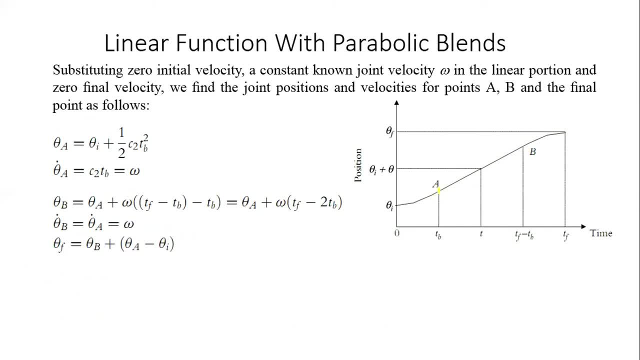 and because, because we know that acceleration in this period and in this period is constant and the acceleration in these two periods are same. so we can say that theta f equation at this point minus theta b should be equal to theta a minus theta i. so this expression has been written in this form. take derivative of this expression, you will get. 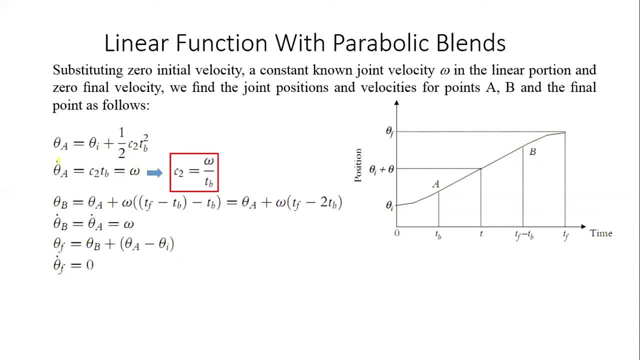 theta f, dot is equal to zero. and just simplify this equation and this equation gives: c2 is equal to omega by tb. and simplify you this equation: using this equation and this equation we get: theta f is equal to theta i plus e to t b square plus omega e of minus 2 tb. put c2 is equal to omega by tb and we 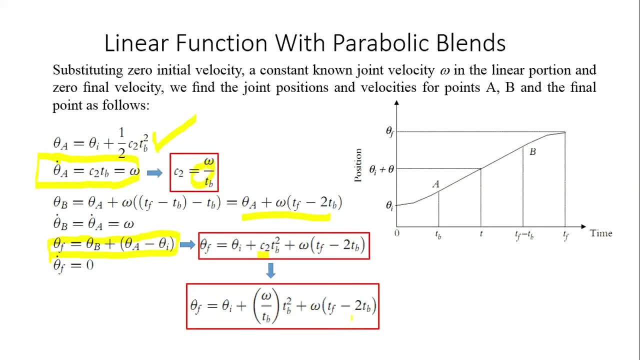 get theta f is equal to theta i plus omega by tb into tb square plus omega tf minus 2 tb. so this equation can be simplified for obtaining the time tb and the expression of tb will be equal to theta i minus theta f plus into t of omega, this constant velocity into total time t of divided by constant velocity. 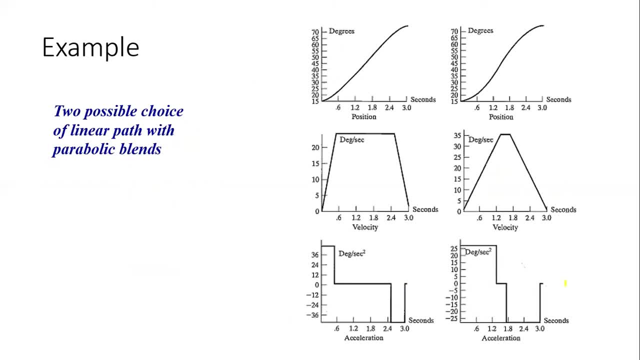 omega. Now take two possible choice of linear path with parabolic length, and in this we have taken a smaller blend, a blend with smaller time period, and in this case the blend is taken for a longer period of time, So the constant velocity in this case is for larger period of time and in this 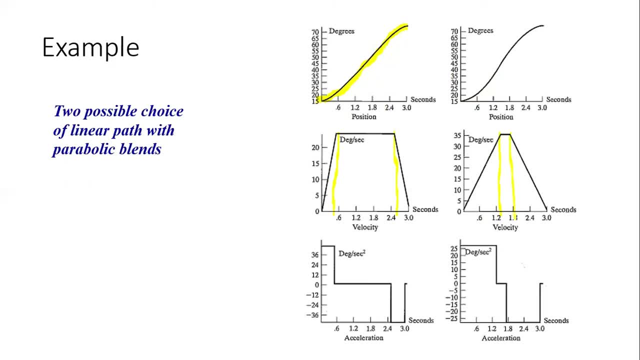 case it is for smaller period of time. So if we take its derivative of velocity, then acceleration profile will look like this and you can see that acceleration is applied for a smaller period of time, but the magnitude is higher as compared to this profile. In this profile, a smaller acceleration 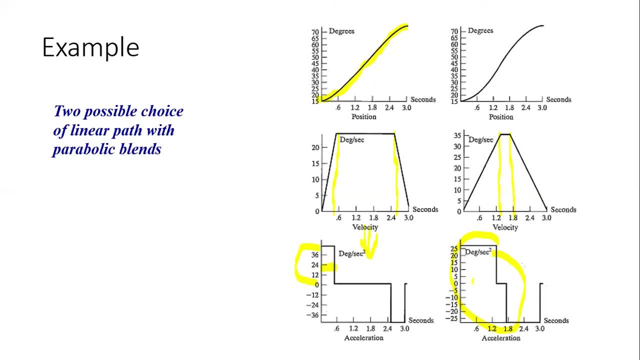 has been applied for a longer period. So if the motor is capable of producing a smaller torque or a smaller acceleration, then we can say that the velocity is applied for a longer period of time. should use this type of trajectory and if there are, there are no limit of acceleration or torque. 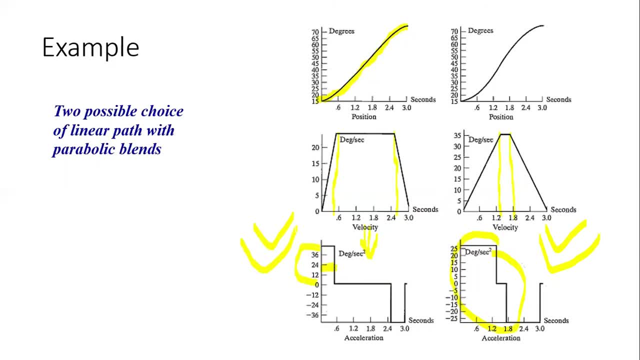 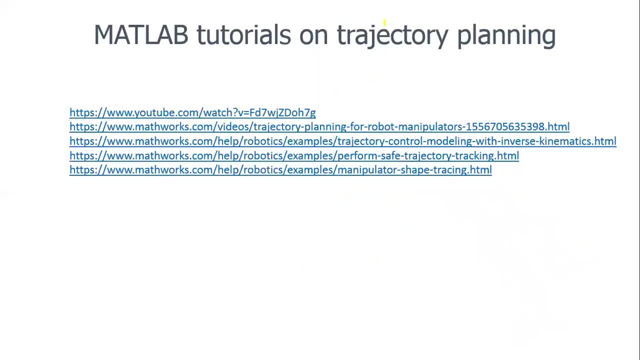 produced by the joint, then we can use this type of trajectory. so as for the requirement, we define the trajectory of the robot so you can use these youtube links for understanding the trajectory planning from matlab point of view in matlab framework. so some lab tutorials are given in: 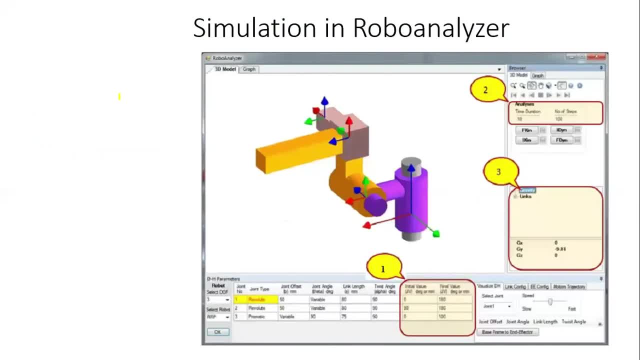 these youtube links. you can also analyze the trajectory planning concept in a robot, in different robots on robo analyzer platform, and for that you need to follow the following steps. so first of all, select any kind of robot and define the ds parameters for that robot. in this, 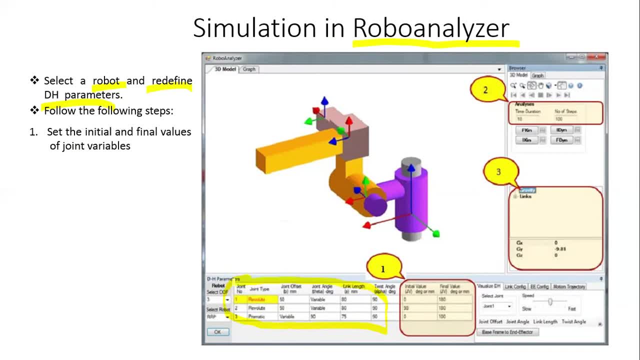 space, then follow the following step. the first step is to in is to define the initial and final values of joint variables so you can define the theta initial and theta final. then set the time duration and the number of steps in which you want to simulate your behavior so that can be assigned in display in this space. then set.